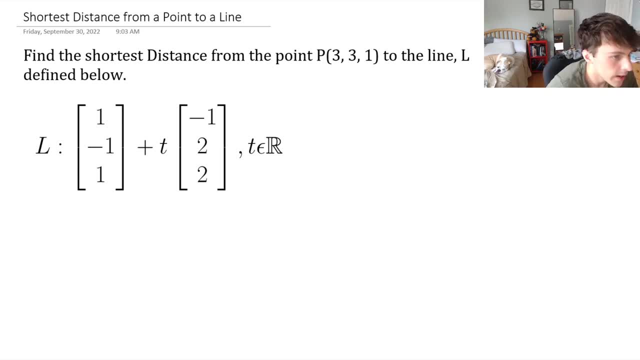 In this video we're going to be looking at how to find the shortest distance from a point to a line. The first thing I do when I want to start off a question like this is always just sketch it out. I think it makes it a lot easier to understand what you're doing. 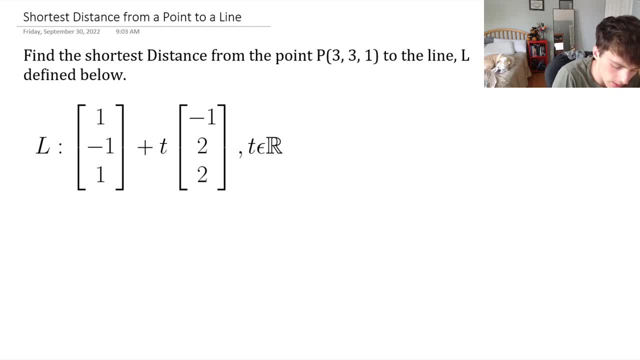 So let's start with what we're given. Let's just draw some arbitrary line and we'll call that L, And we'll label this with all the information that we know We'll call this L And we know that it has a direction vector. 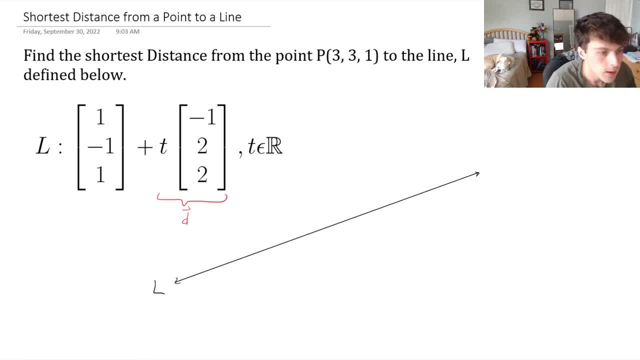 We'll call this D of. So let's just draw some arbitrary vector here, This red vector. we'll call that D, And we know that it's in the direction of the line. And we also know that it's in the direction of the line. 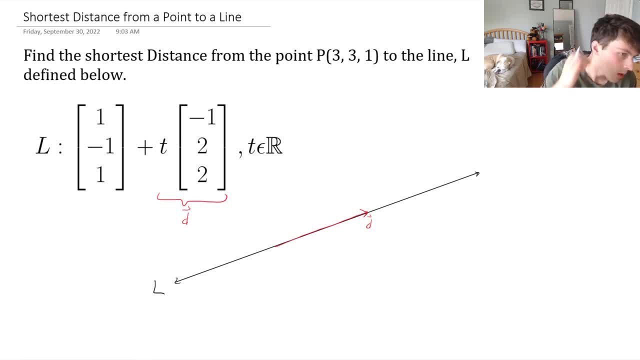 And we also know from the equation of the line that would be a point on the line. And to check this, plug in: T is equal to 0. And you can see that the point would be on the line. So let's just draw an arbitrary point on this line right here. 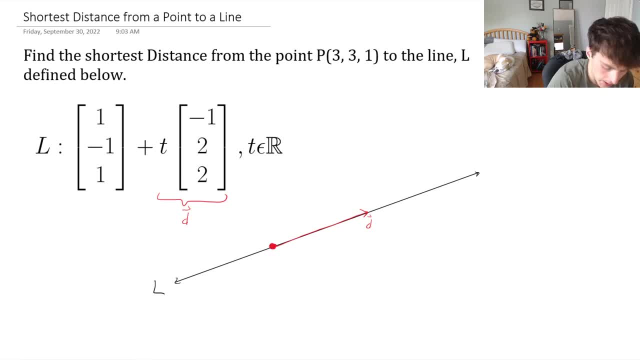 And we're going to label that as: And we're going to label that as P, P0, or P0.. Remember, that's a point, not a vector. And then we've got direction vector D. Now we are looking to find the shortest distance from the point to the line. 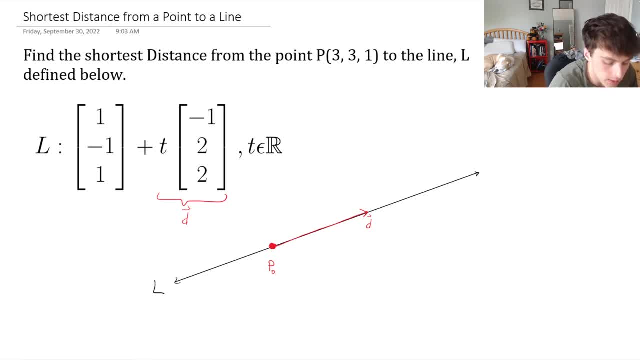 So let's just label some arbitrary point in this little sketch, Let's put it right over here And we'll call this P, which is- And we're just playing with a random point here. We don't know where exactly things are, but we're just going to put everything into a diagram. 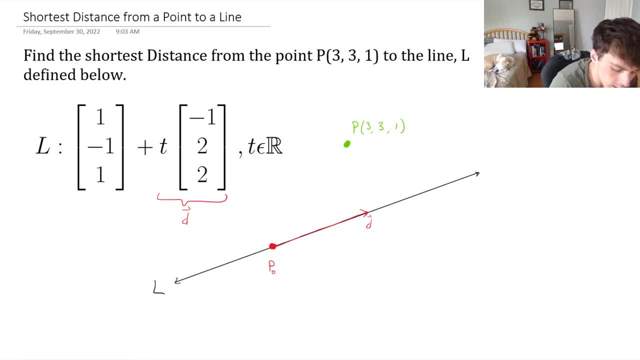 So the process to solve these questions is not too bad. The first thing that we want to do is come up with a vector That goes from point P0,, which is a point on the line, to the point of interest, which is point P. 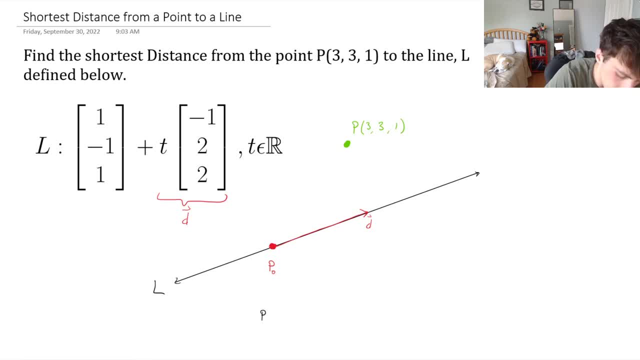 And we can do that by doing: Well, let's create a vector P0 to P, And we know that this would be equal to the vector from origin to P, subtracting the vector from the origin to P0.. So let's sketch that out to make it make a little bit more sense. 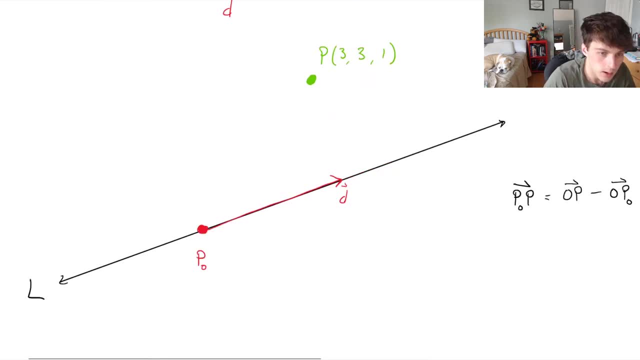 Let me rearrange this a bit. Okay, so let's label some arbitrary origin on this little diagram we've got. We'll call this the origin right here: 0 or O, And let's just see, because a lot of people get confused when they do this calculation. 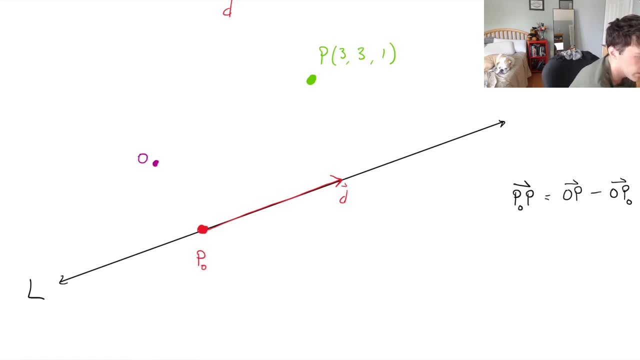 They just do a point P and they subtract the point P0, and then supposedly that gives them a vector. But that's not true. Remember, when we're trying to get this vector from P0 to P or from the point P0 to P. 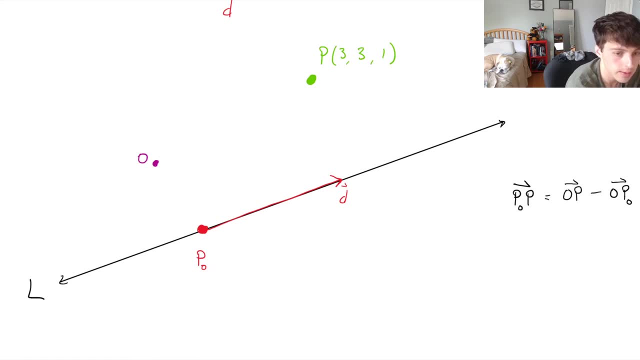 we need to subtract two vectors to get that vector result. Subtracting points will not get you anything. We need to do vector addition and vector algebra here So you can see if we were to draw a vector from the origin to P in purple there. 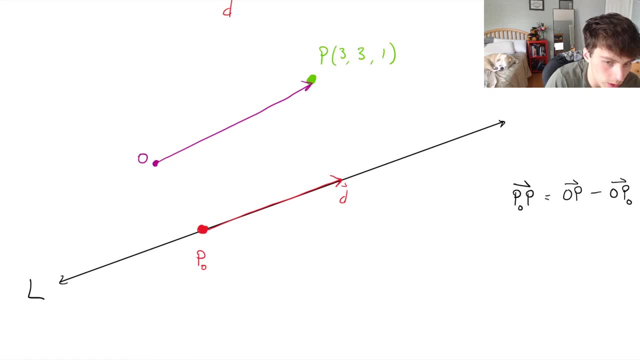 and let's do another one here, The origin to P0, that'll be something like this, And let's actually change the colors here: Origin to P is going to now be purple, and origin to P0 is going to be orange. 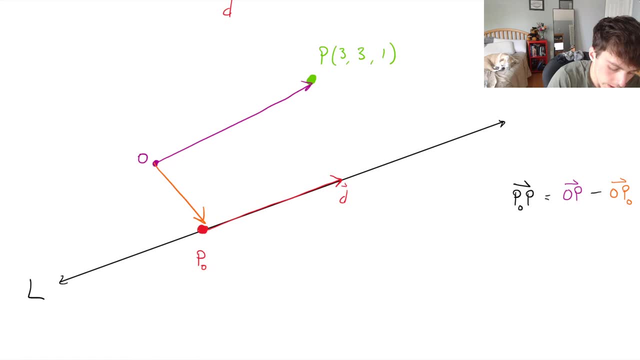 Great. Well, we can see that if we were to do origin to P and then plus the negative vector, origin to P0, well that would just be like adding the origin to P0 from the other direction. So the result would be a vector that looks kind of like such right. 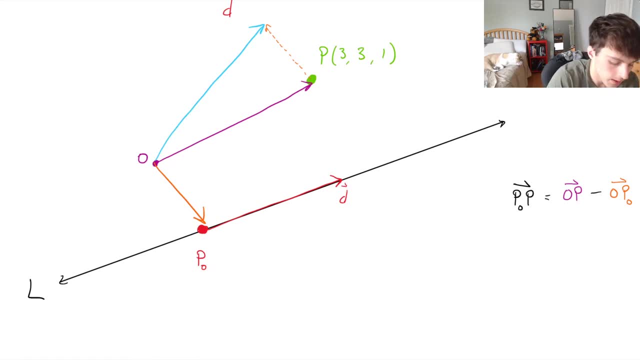 And this is going to be in blue right And you can see if we were to shift this just down and to the right. you can see that this vector right here results in from P0 to P Right. So let's actually do this math. 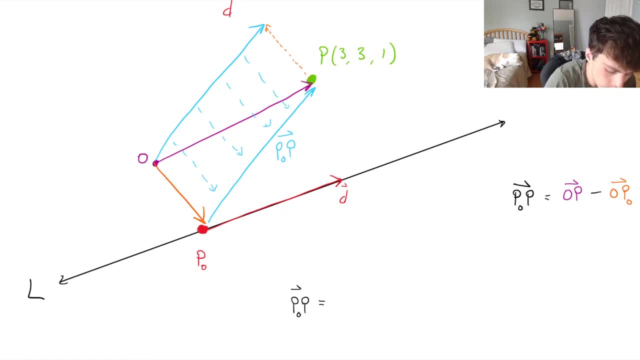 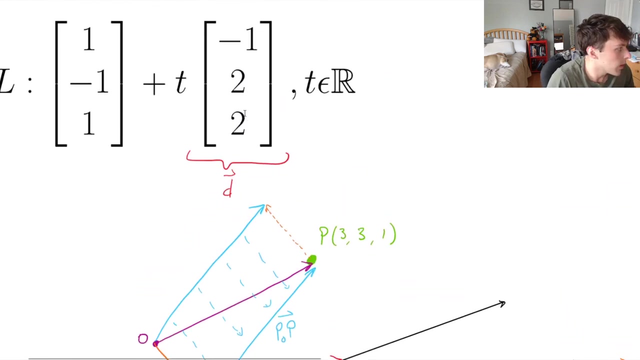 P0 to P would be equal to well, from origin to P0,. we know that that vector is represented by, and we're subtracting. well, the vector from the origin to P0, is represented by, and the point we had was right. 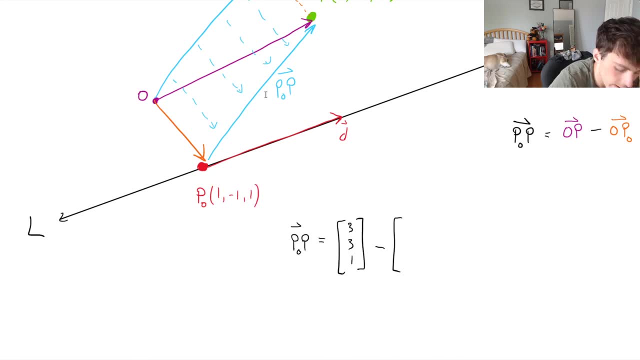 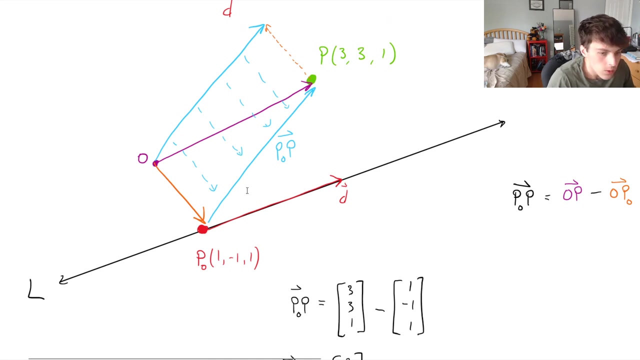 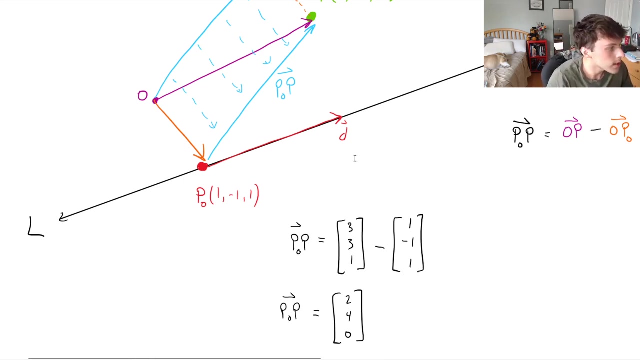 Let me just label that Great. So we know that this vector now is going to be Great. Okay, So what next? Well, we're looking for the shortest distance, right, And the shortest distance we would know. 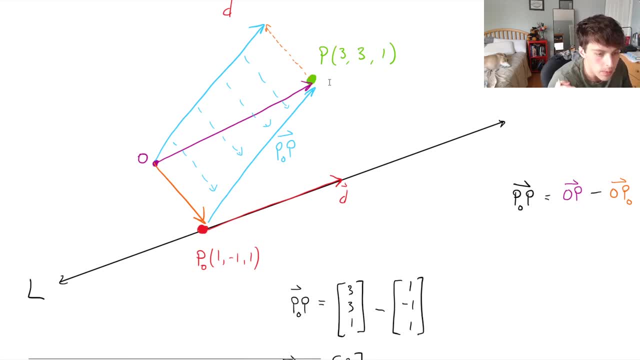 is going to be the perpendicular distance from the point P to the line Right. It needs to be perpendicular. That will result in the shortest distance, And we know that a perpendicular line would look something like this, Approximately like this: Right. 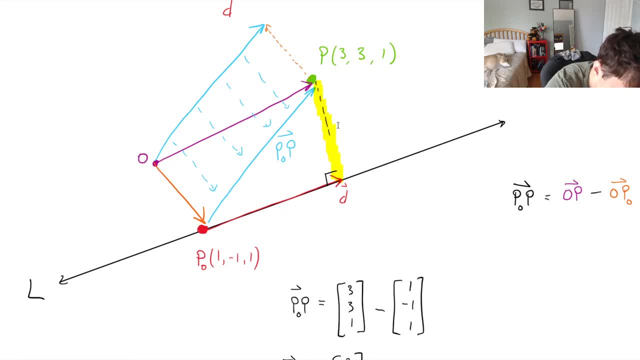 And you can see that that would make a right angle here, Right, And what I want you to notice here is that, well, this is just the perp of P0, P onto the line with direction vector D. Okay, So let me label that. 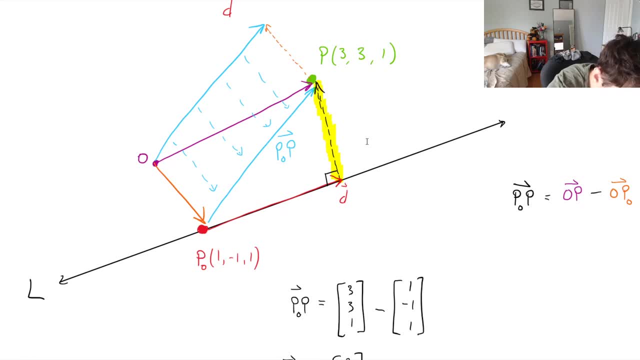 You can see right here, if I were to make this a solid line right, draw it as a vector. Well, this is by definition the perp of P0 to P onto the direction. vector D, Right, Makes sense. 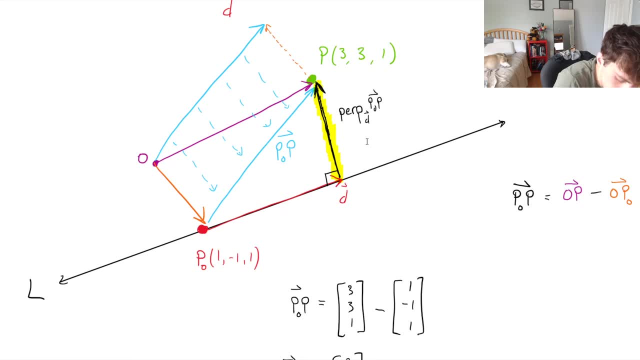 And here let's shift this just a little bit. this direction, vector D. And we can see that, this, oh, we can see that this line. let's draw running out of colors here, but here I'll just do a more bolded black line. 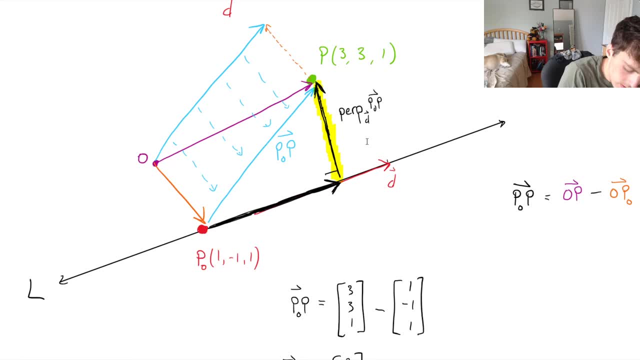 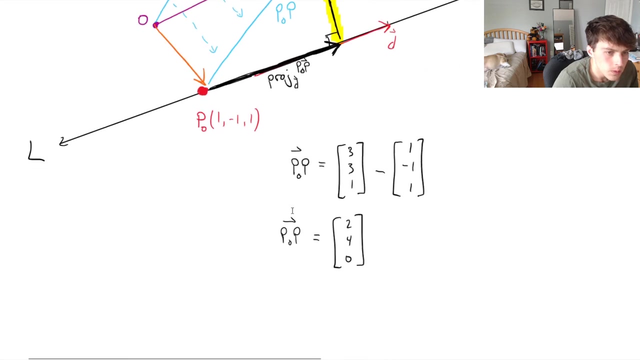 You can see now that this right here. well, this is going to be the projection of that blue vector P0 to P onto the direction vector D Right, Because this line has the direction of D Right. So it'll be useful to find the perp. 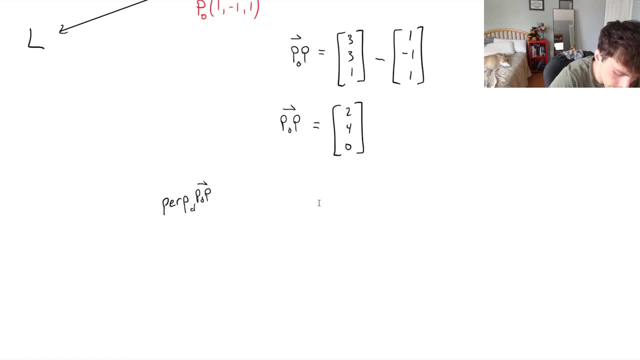 of P0 to P onto the direction vector D, And we know that this is just going to be equal to P0 to P, minus the projection of P0 to P over D. Right, And you could, I encourage you to do the same thing. 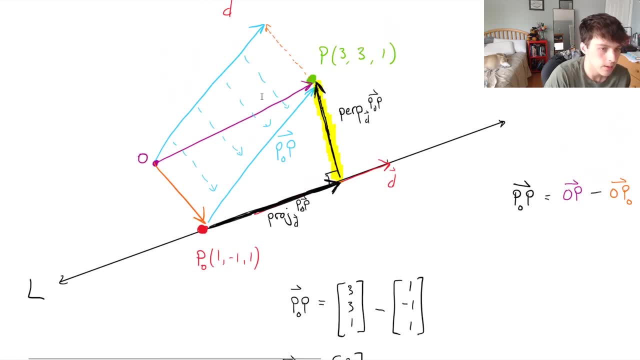 that we did above with this blue vector when we did from origin to P, this purple vector plus the negative of this orange vector, and we resulted in this blue vector here. I would recommend you doing the same thing with this equation to see how this makes sense. 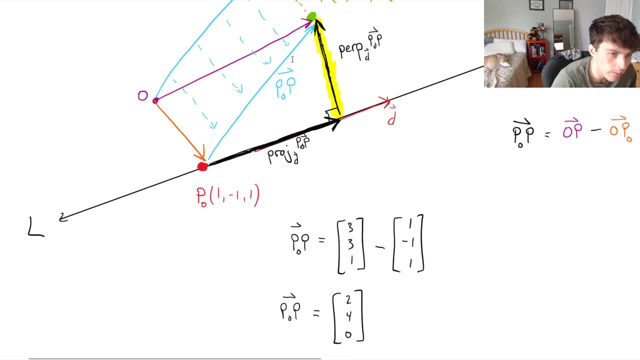 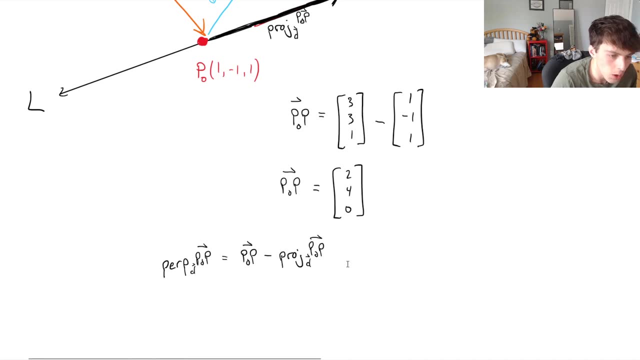 because these are all just vectors and we've already gotten them written down all here. So if you did the same sort of approach, you would see that all these vectors should make sense in your head. why this addition and subtraction works. So let's now just 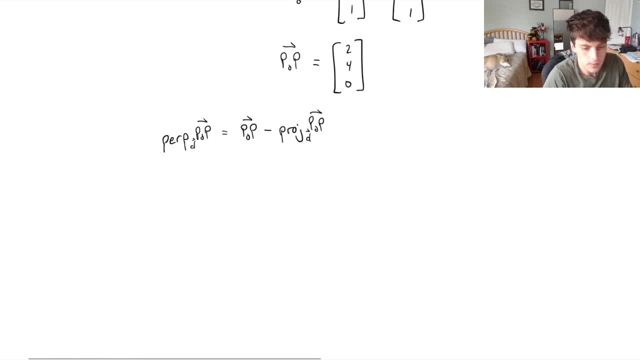 let's calculate this vector right. So we have 240 minus. well, projection formula: we know this is P0P dotted with direction vector D over magnitude of D squared, and it's in the direction of D. Okay, This will be 240 minus. 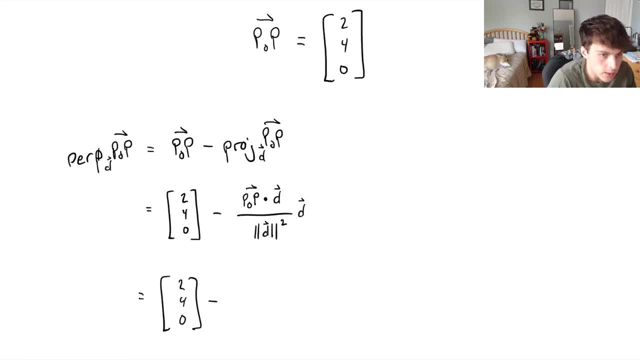 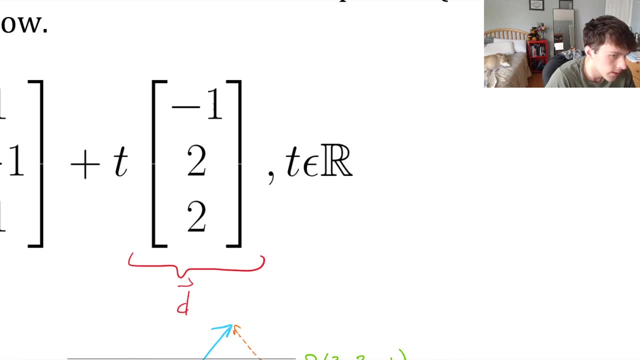 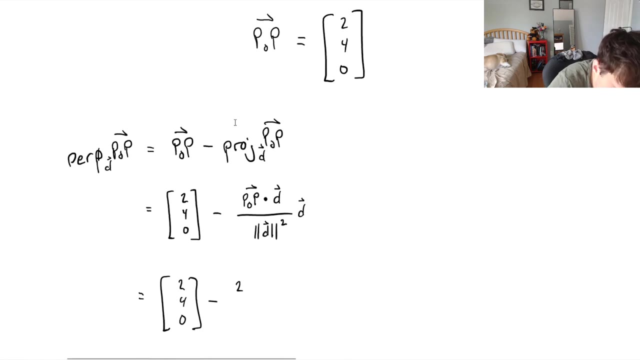 okay, P0P is dotted with D, So it's 240 and our direction vector D is negative. one, two, two, So this will be two times. actually- let's put these in brackets- two times negative, one plus. 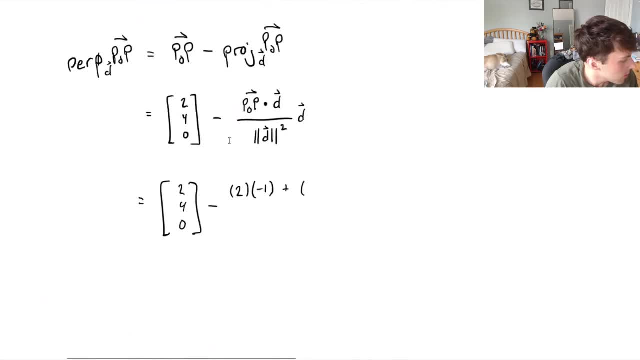 oh, I've already forgotten. negative one, two and two. Negative one, this will be two, and this is times four plus and this will be zero. And now we've got to do the norm squared. So the norm squared is just going to get rid of. 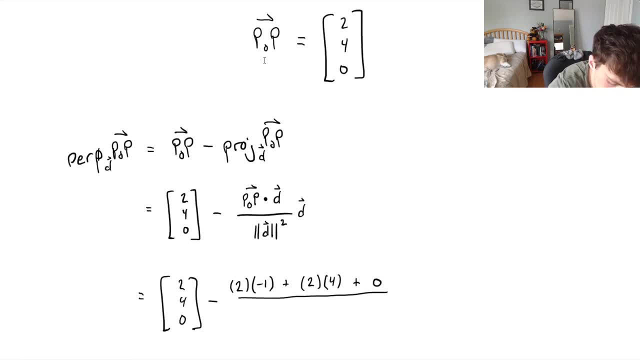 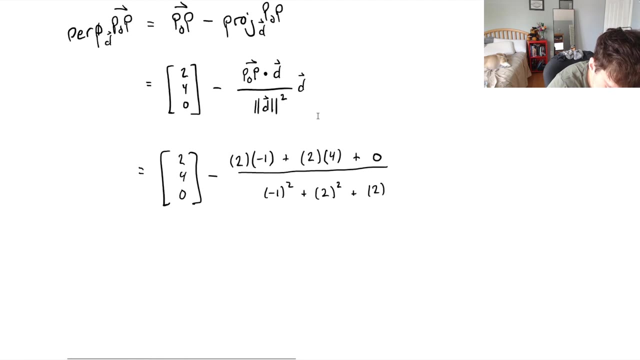 the square root and we're going to square all of the terms. So this will be negative. one squared plus, two squared plus, and double check here: yep, two Great, And it's in the direction of negative. one, two, two. 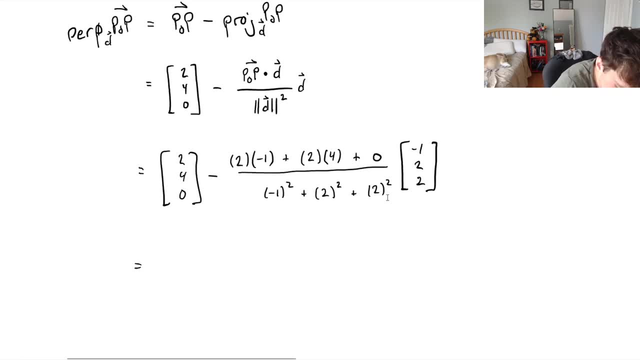 So let's just clean this up. do some quick math: 240 minus, and this is okay, negative two plus eight is going to be six over. this is one squared plus four plus four, so that's eight. So this is going to be nine. 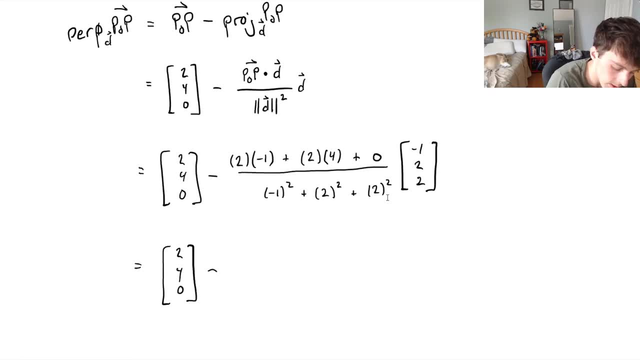 We've got six ninths, which is just two thirds. right, And this is negative. one, two, two, And let's express this as one answer. We've got two now. we've got now two plus two thirds, So that'll be six thirds plus another two thirds. 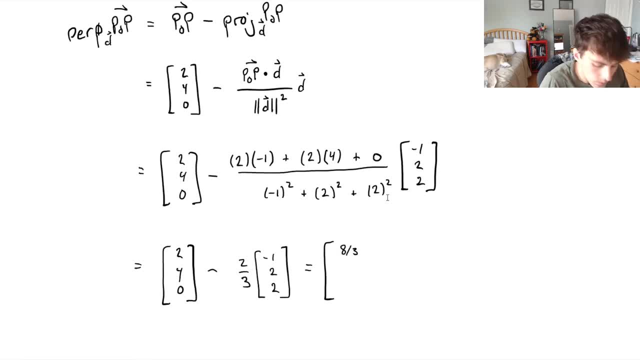 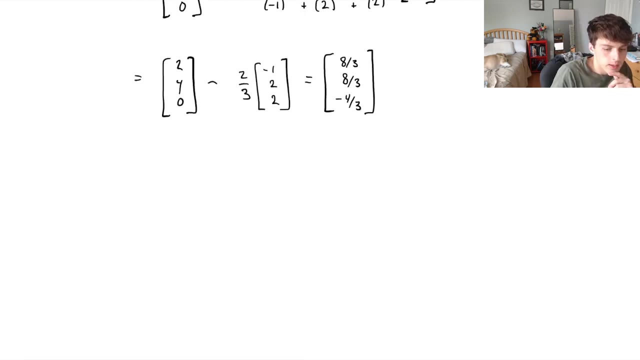 so that'll be eight thirds Four minus four thirds. Well, oh God, So it's getting a little bit uglier here. For sake of time, I'm just going to do this math and get the answer in one sec. 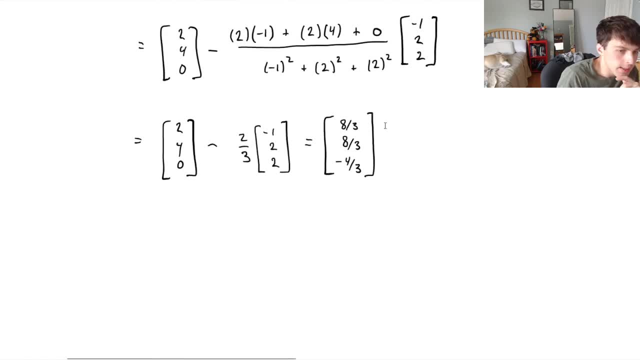 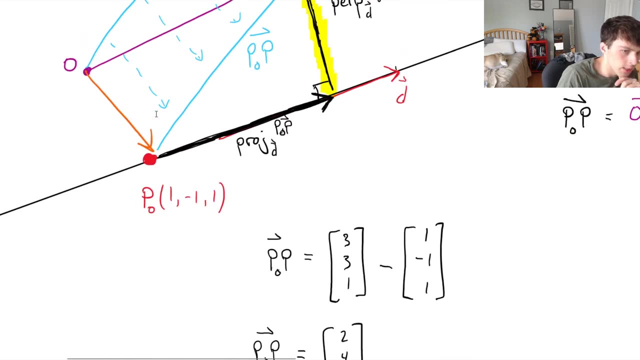 So, doing a bit of quick math, we get this vector here And remember, this is the perp vector of P, not P onto the direction vector D. So this is this highlighted vector And this we're looking for the shortest distance. 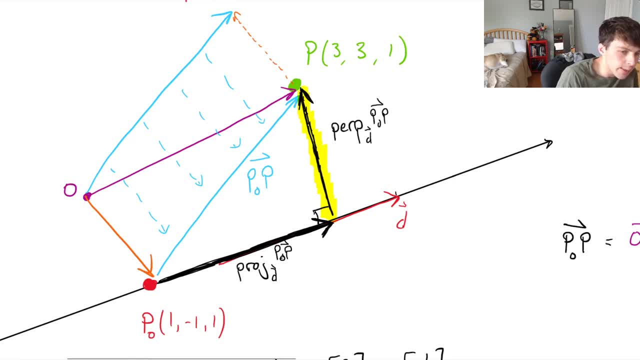 but remember, the shortest distance is not a vector, it's a length, right? We want the length of that vector, So really we want the norm Of this vector, So we actually have to take the norm of this. 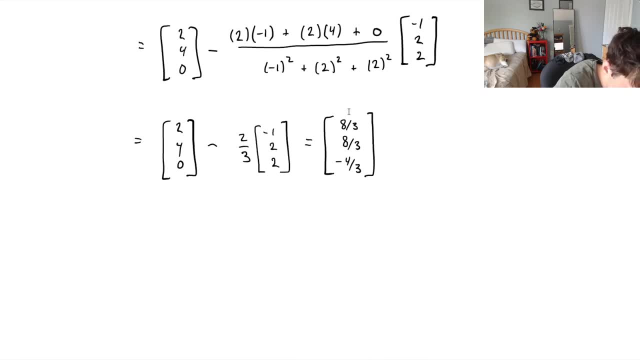 right. So that's right now the norm of perp, of P, not P, onto the direction vector D. That's going to be equal to the square root of eight thirds squared plus eight thirds squared. Minus, oh, plus, sorry. 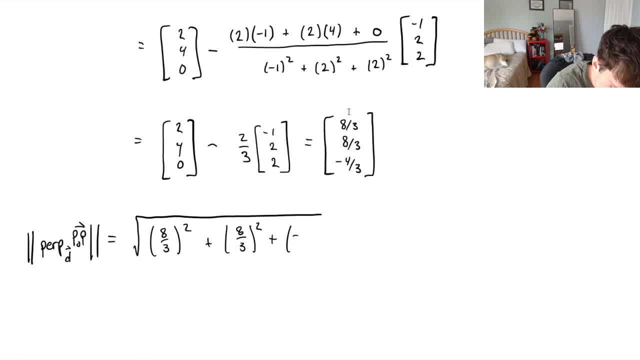 minus four thirds squared. Doing some quick algebra, we know that we've got a common denominator of a third in each of these terms, So we can pull out a third squared and then we would get one third squared on the outside times. the square root of 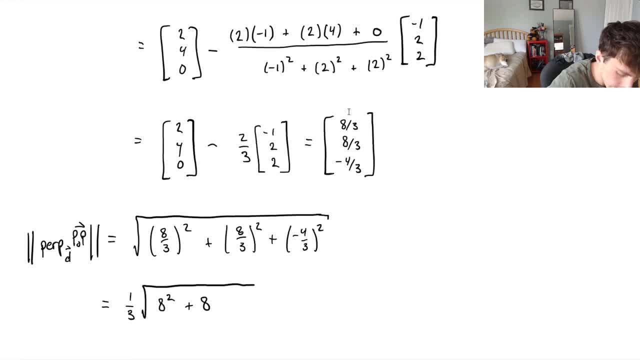 this will be eight squared plus eight squared plus negative four squared, which is going to be 64 plus 64 plus 16.. So 64,, 64, and 16.. If we don't have a calculator, like we don't right now, 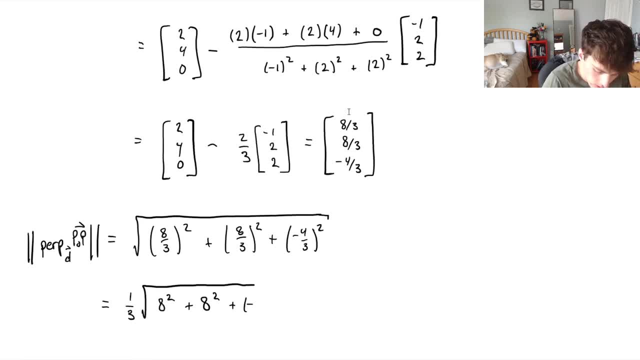 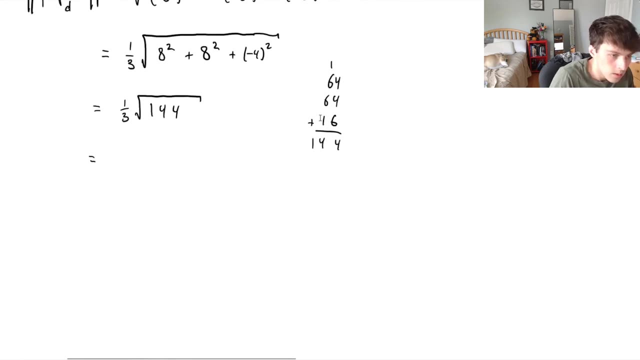 I'm just going to add this using fundamentals: We've got 14,, six, 12,, 13,, 14, we get 144.. So that's going to be 12, right, Yeah, makes sense to me. 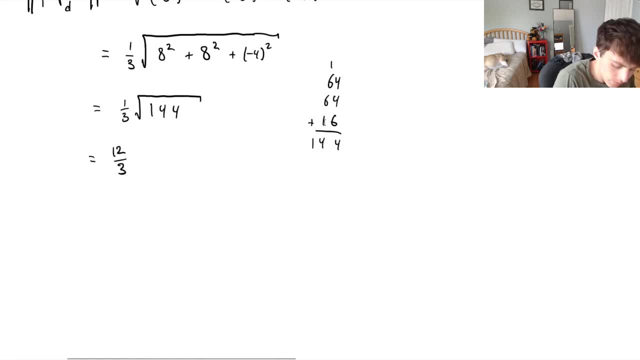 So we would get 12 over three, which is just going to be equal to four. So the shortest distance from the point that we were given to the equation of the line that we were given is going to be a distance of four. 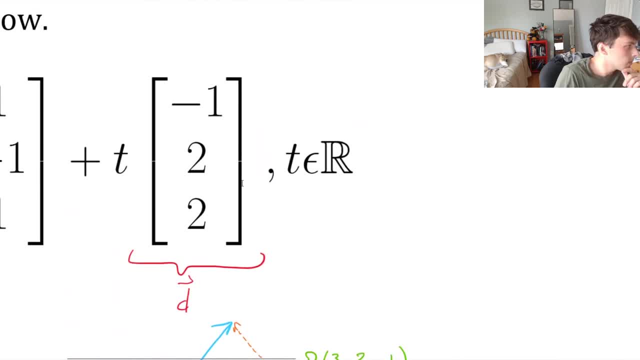 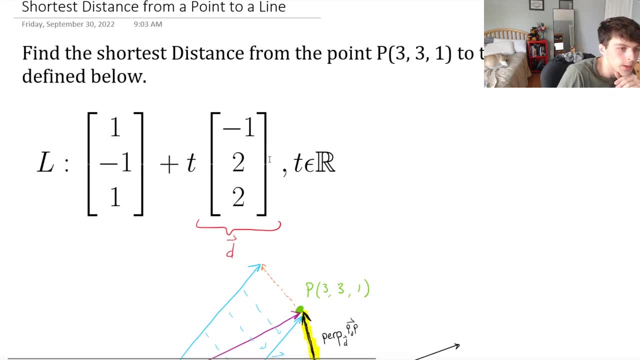 Right, So this distance right here is going to be four, And that's it for this question. Yeah, I hope this was helpful And yeah, drop a like. Thanks.